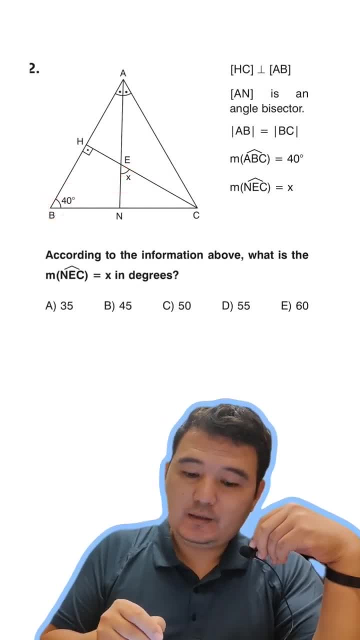 Let's find the X in the problem. We have 40 degrees here, an angle bisector, 90 degrees over here and equality of sides AB and BC. So AB is here and BC is here. So this is isosceles triangle. 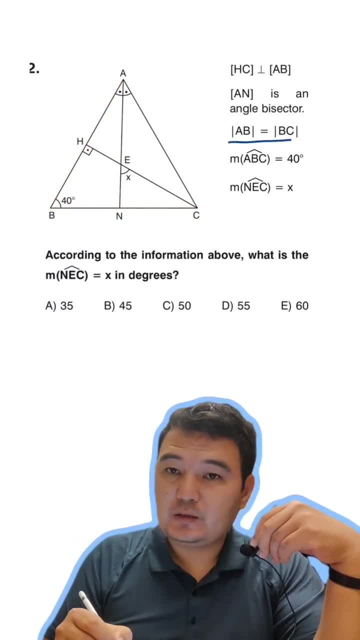 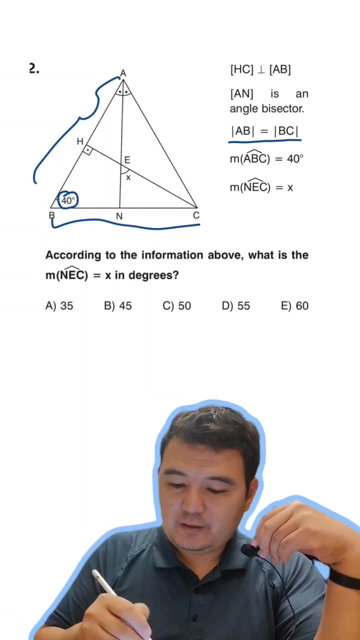 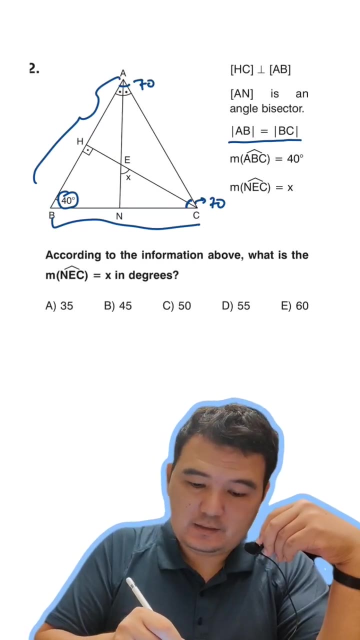 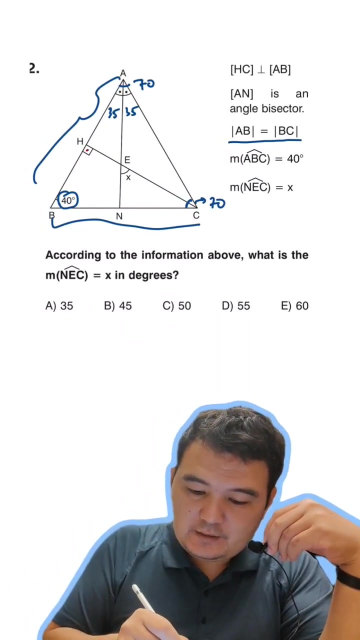 So, first, if you start with this equality of AB and BC, so this and this, since the the measure on the top is 40 degrees, the measures here should be 70 and 70. So which makes these angles 35 degrees each. The other side of this, 90 degree, is also 90 degree. So now looking at this triangle. 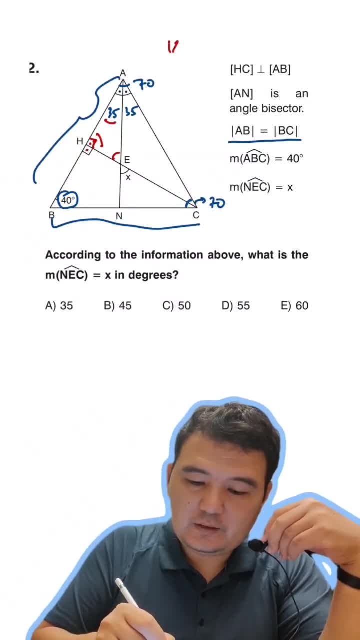 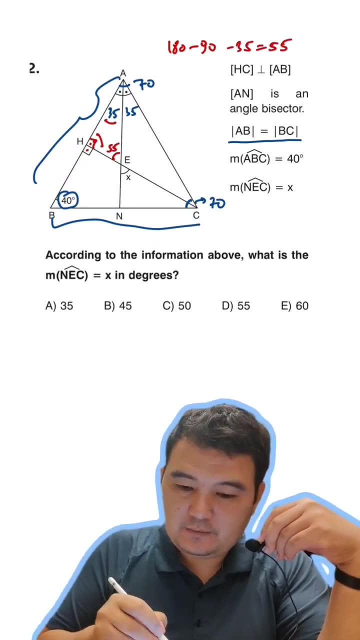 you can say that 90 plus 35,, 180 minus 90 minus 35 is 55 degrees, So this is 55.. And now X and 55 are vertical angles, They are equal to each. 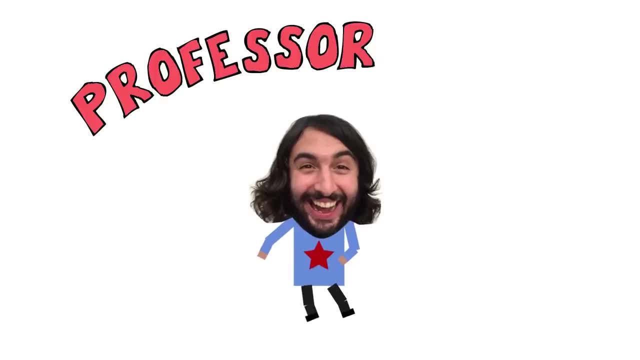 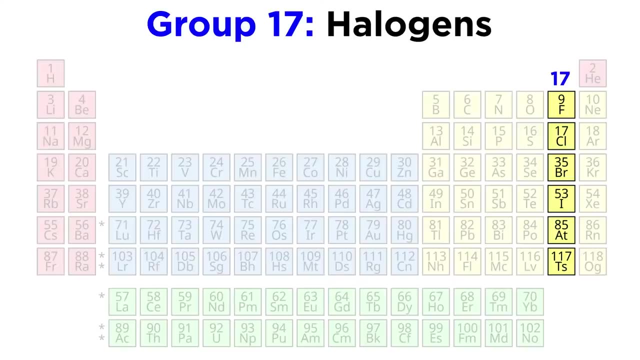 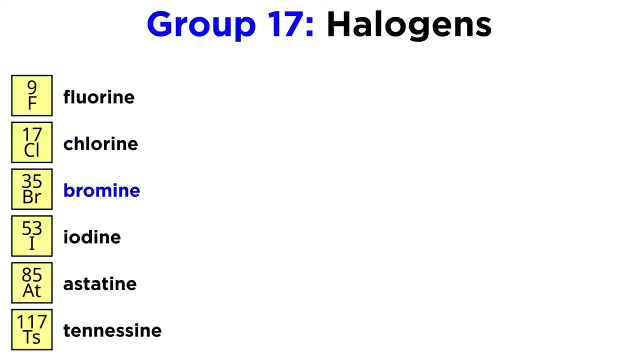 We are almost at the end of the p-block now, having arrived at group 17,, which are known as the halogens. This group includes fluorine, chlorine, bromine, iodine, astatine and tenosine. All but the last two of these elements should be extremely familiar. 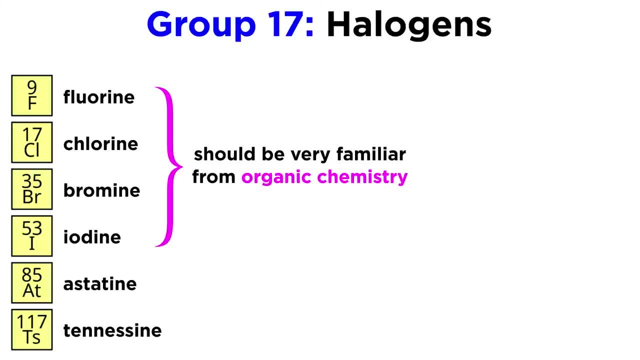 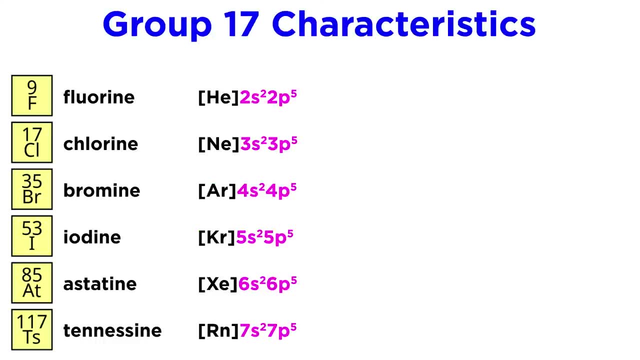 from organic chemistry, as these first four are ubiquitous in organic synthesis. All of the halogens are nonmetals and they have very similar properties. They all have electron configurations ending in ns2 and p5, which means they have a strong tendency to gain. 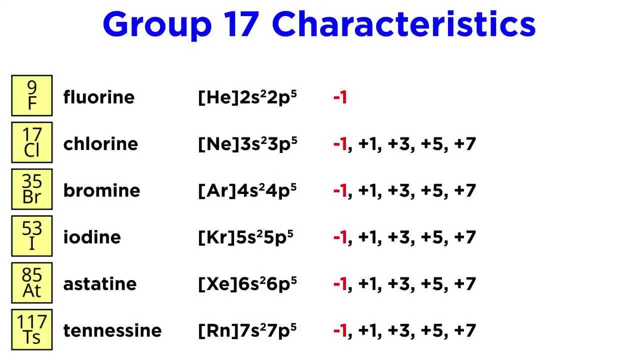 one electron to complete their outermost shell. Thus the minus one oxidation state is very common for these elements and is the only oxidation state fluorine will attain, while the others can also be plus one, plus three, plus five or plus seven, depending on what they are interacting.